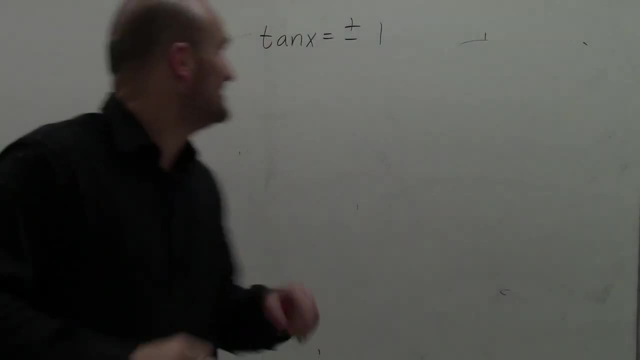 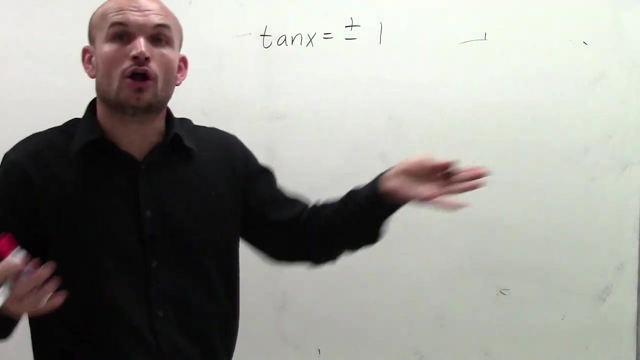 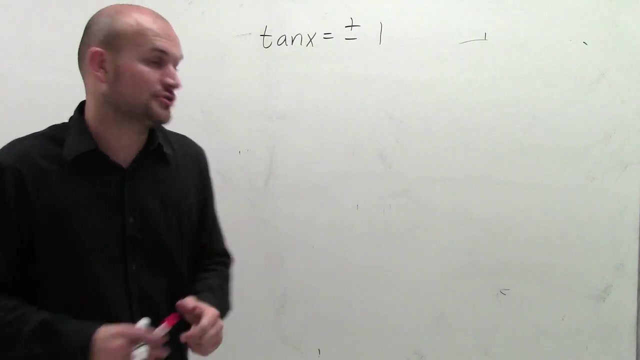 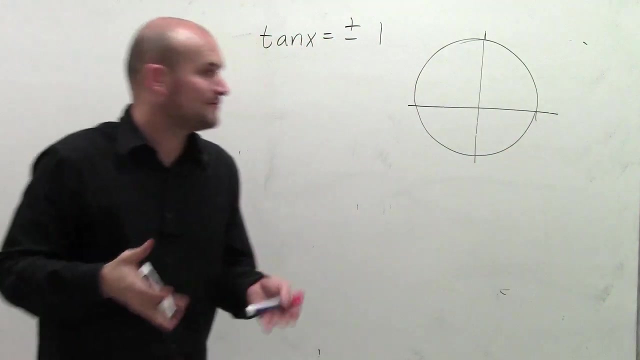 Hello. So what we have is tangent of x equals plus or minus 1.. And what I want to do is show you how to write all of the solutions, for all the solutions of tangent equals plus or minus 1, and not only just the solutions on an interval of 0 to 2 pi. So the first thing we want to do is actually just find all the solutions on the interval of 0 and 2 pi, So therefore we can rightfully actually figure out what all the solutions are going to be of the graph. So the first thing, when tangent equals plus or minus 1,, 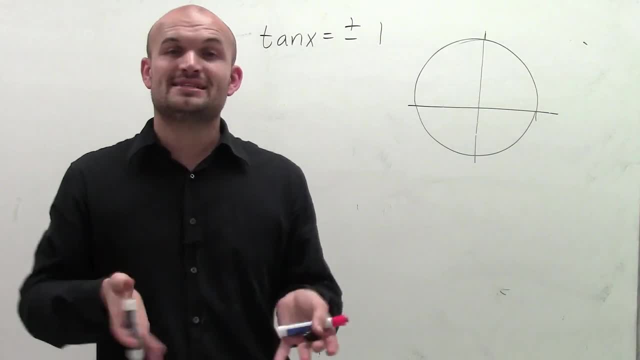 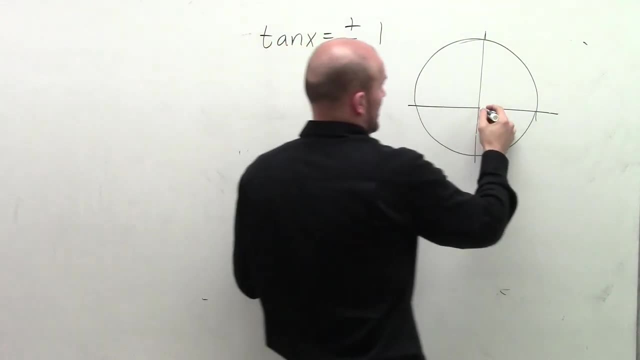 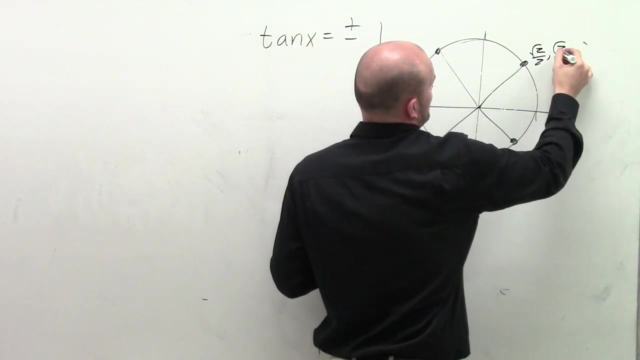 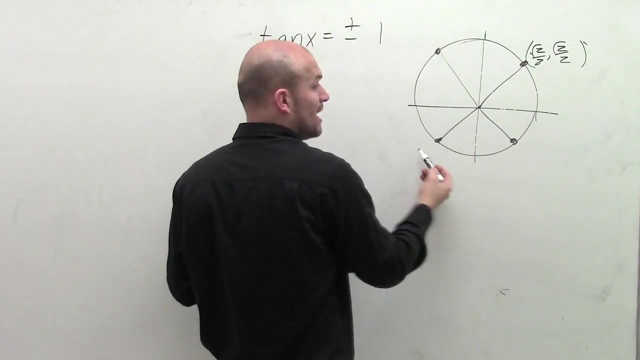 remember tangent is on the unit circles, when we take our coordinates, our y-coordinate over our x-coordinate. So there's four angles or four solutions that we're going to have for this problem on the interval of 0 and 2 pi. And I'm not going to write over all of them because you can see, all these are just reflections, which now the x being negative, the x and y being negative, and here the y being negative, But our angles are going to be pi over 4.. 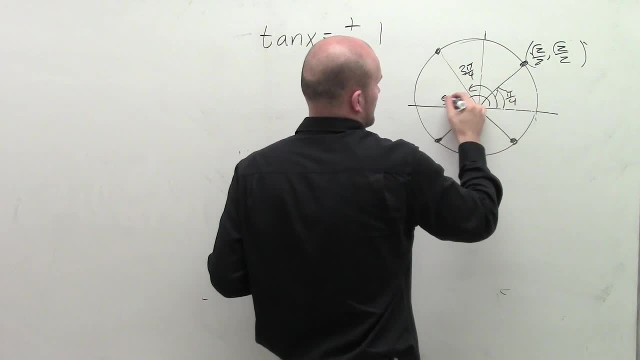 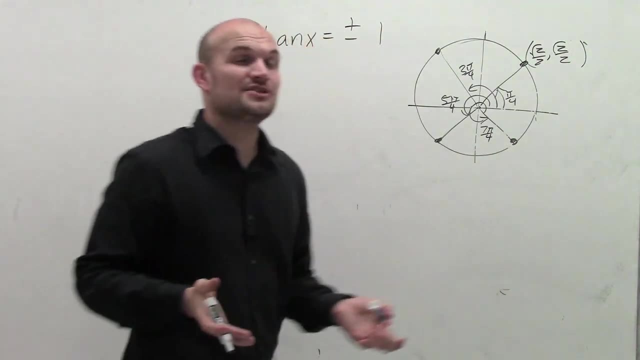 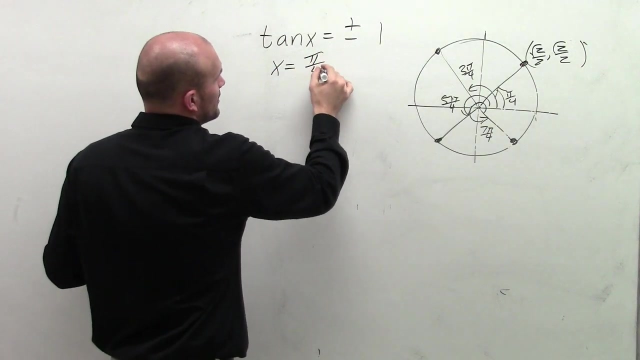 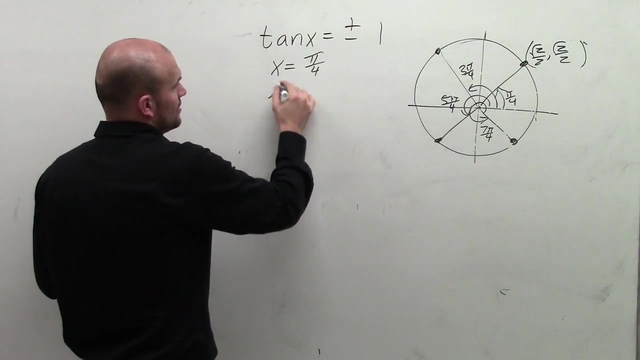 3 pi over 4,, 5 pi over 4, and 7 pi over 4.. So if I was going to ask you to find all the solutions on the interval of 0 and 2 pi, then you would write down those simple solutions And you just say: well, tangent of the angle, when equal to plus or minus 1, is equal to. when the angle is x equals pi over 4, when x equals 3 pi over 4,, when x equals 5 pi over 4.. 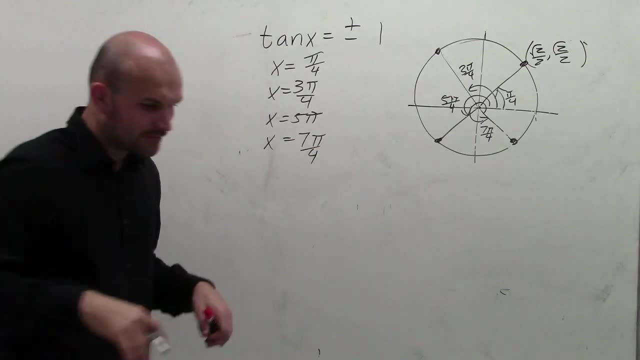 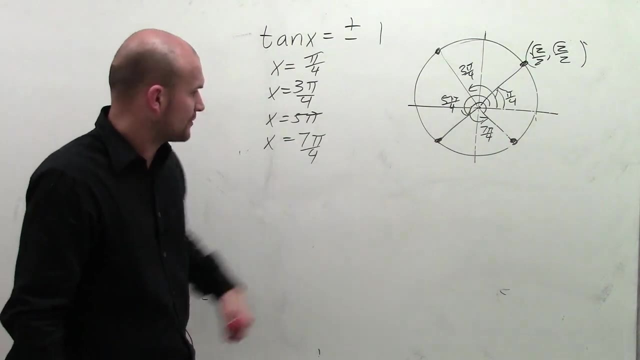 And when x equals 7, pi over 4.. But what if I ask you to find all of the solutions to the graph? And so, to find all of the solutions to the graph, what we're going to want to do is take a look at the graph of tangent. 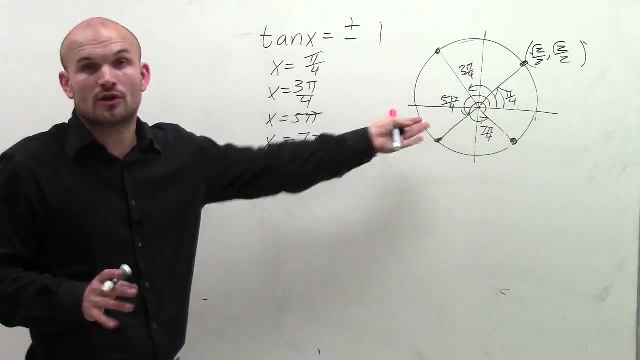 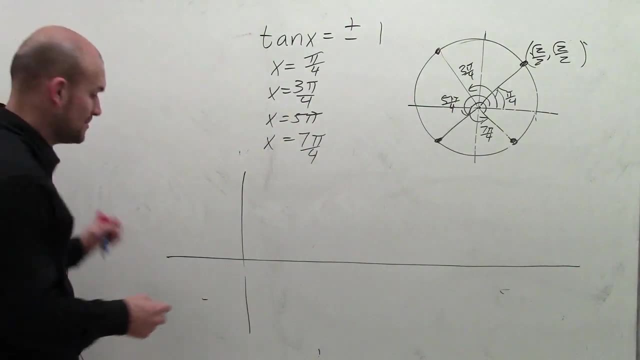 and see how is that going to replicate past our interval of 0 and 2 pi. So let's go ahead and make a nice little graph of the tangent function. So remember, the tangent function starts at the first initial period, at negative pi half. 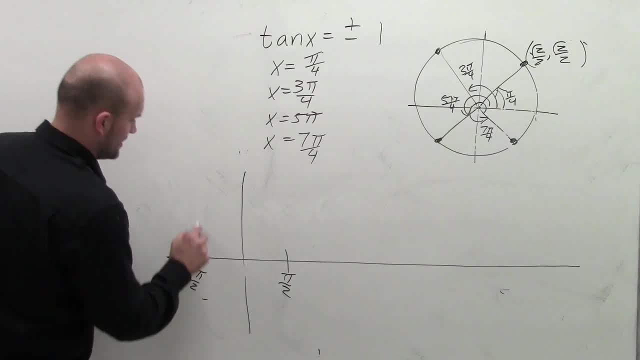 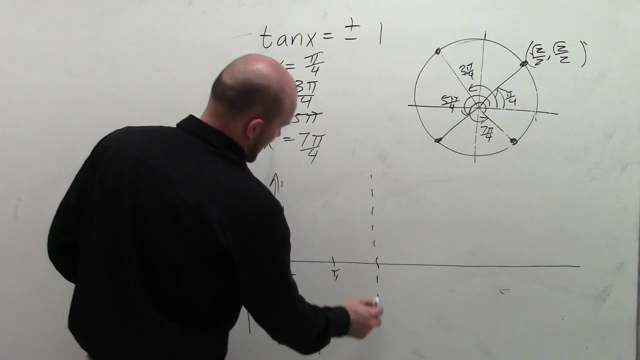 And at pi halves, And then that's where your two vertical asymptotes occur. So then it goes something like this, With a nice little intercept there. So then my next intercept is going to be at pi, And then another intercept at 3 pi halves. 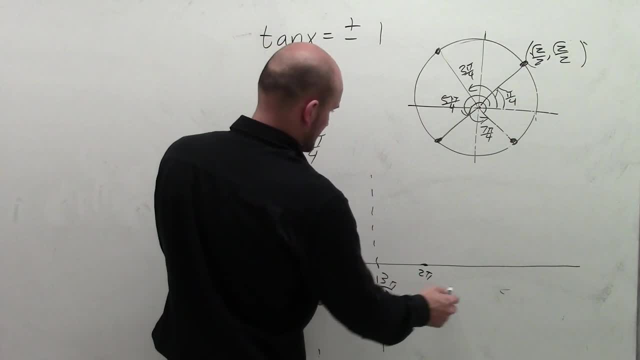 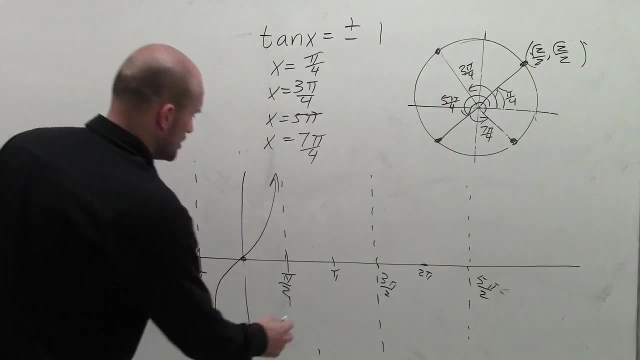 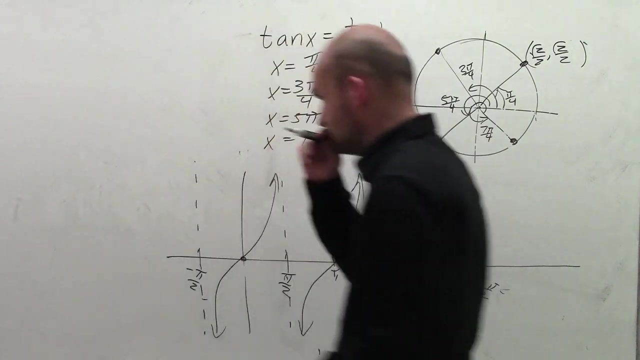 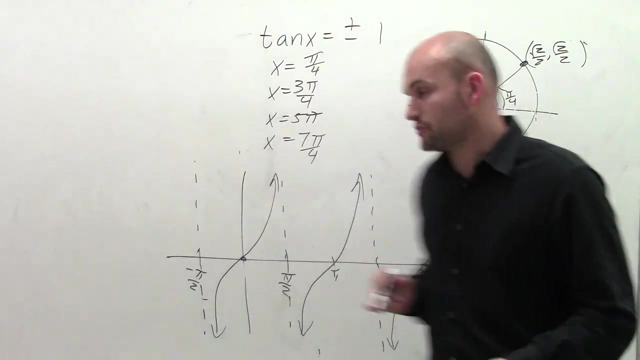 Then I'm going to have another intercept at 2 pi And then another intercept here at 5 pi halves, So it's going to cross here, Looks something like that. OK, So this is what the tangent function looks like. And remember, this is going to keep on repeating, on and on, in the positive and in the negative direction. 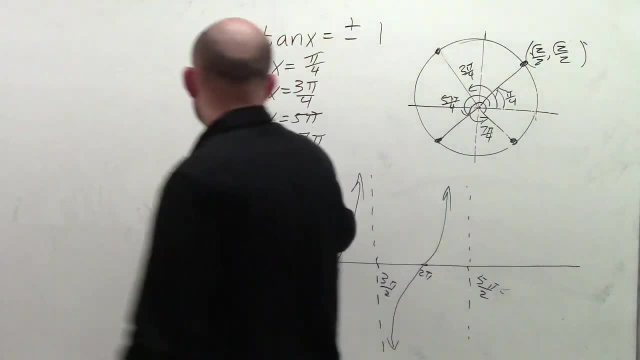 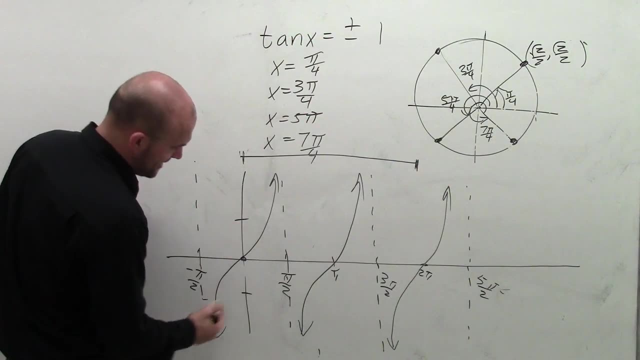 But we said that there's solutions between 0 and 2 pi And there's only four solutions when tangent equaled plus or minus 1.. So when it equaled plus or minus 1 was at pi force, which makes sense. That would be pi force. 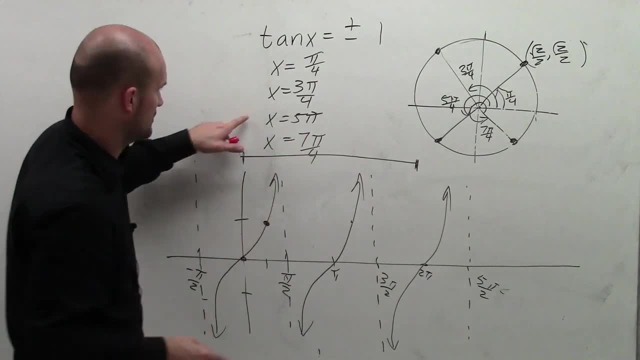 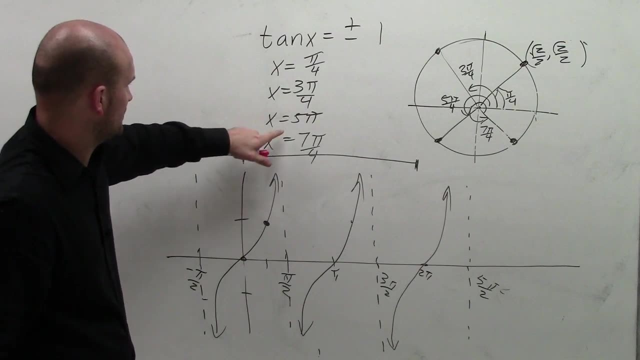 And then also at pi force, And then also not at 3 pi over 4,, but at- why didn't I write that correctly? And then at 5 pi over 4,, which would make sense right there, which is just past 5.. 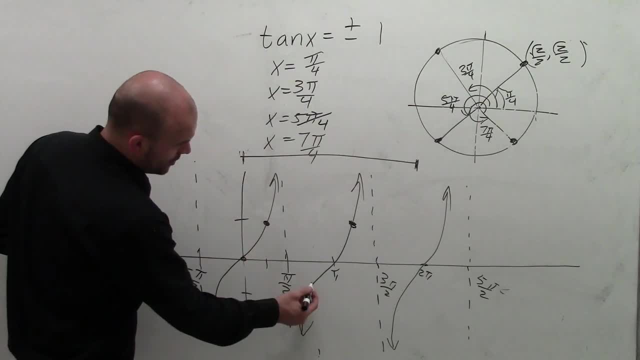 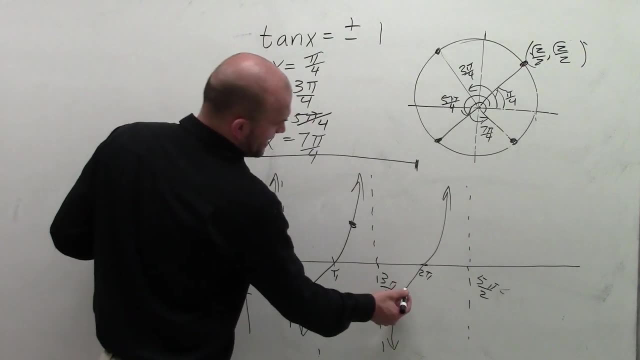 Then it equaled negative 1 at 3 pi over 4.. Let's say so, negative 1, which would be right there, and that's 1. At 3 pi over 4, as well as at 7 pi over 4.. 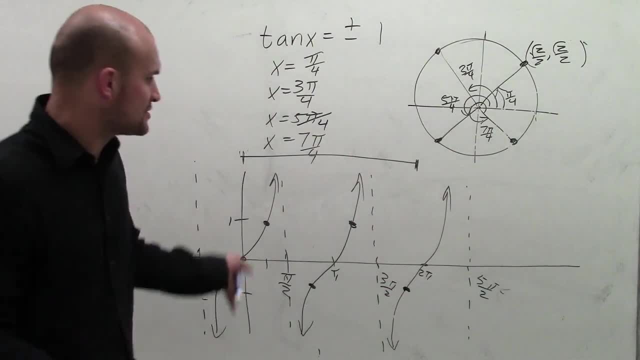 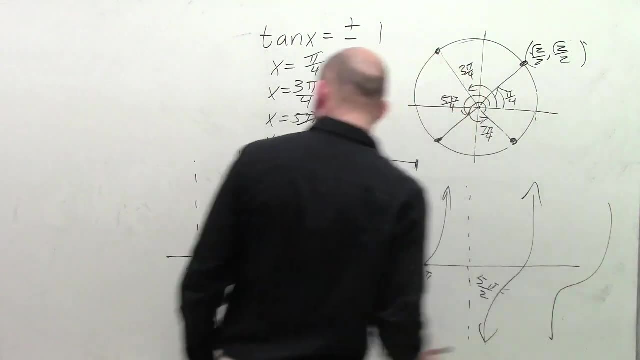 So you can see there are four solutions. Now what about the solutions that are going to continue on outside of 2 pi? What about when I continue my graph going like this or in the negative direction? How am I going to rewrite every single one of those solutions? 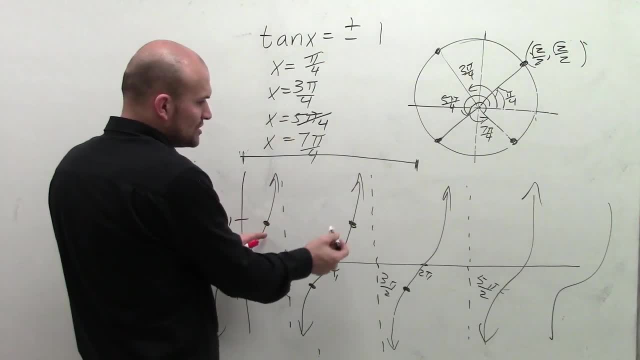 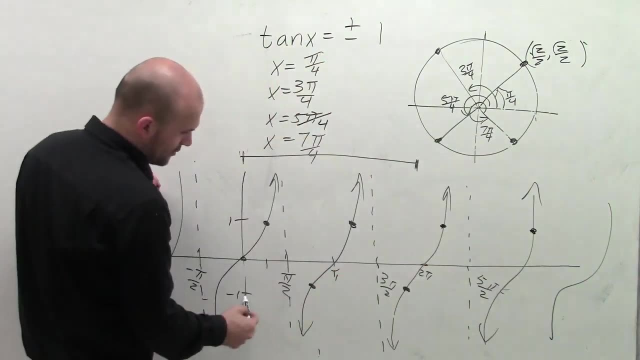 Well, one thing I want you guys to notice is these solutions are going to keep on repeating each other, Because whenever my graph crosses at 1, I'm going to have a solution, Or when it crosses at negative 1, I'm also going to have a solution. 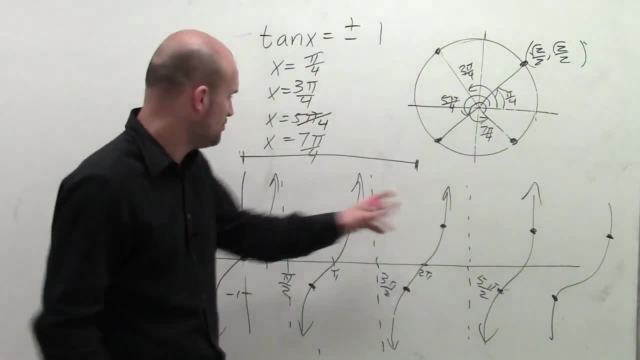 So what I want you to understand is: you can say: well, if I just keep on adding 2 pi, if I add 2 pi to my original answer- pi over 4, that means I'm going to get the next solution. 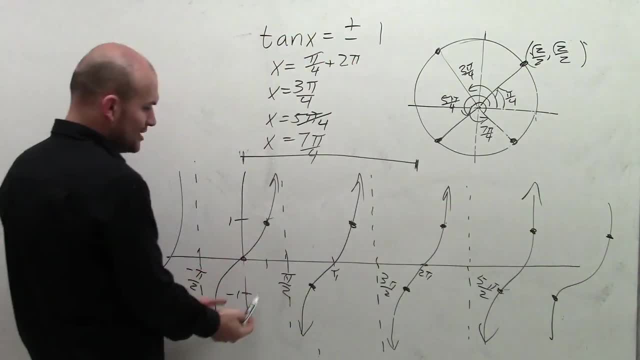 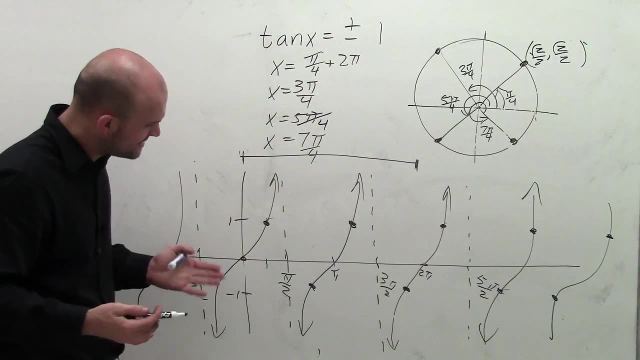 And if I add 2 pi to this solution, I'm going to get the next solution, And you can keep on doing that for all of your solutions, But what's going to happen is you're going to get redundancy. And what I want you to understand is if you look at, let's take the distance from this solution to this solution, 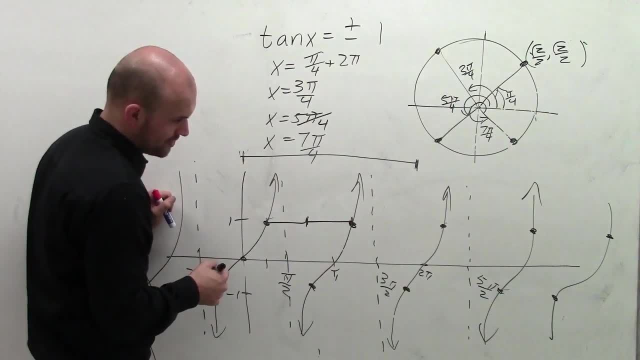 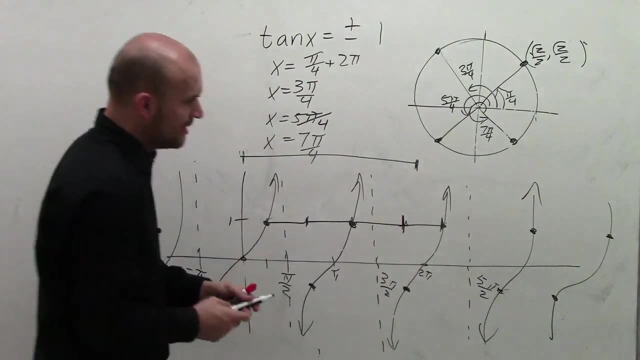 Then let's take a look at the distance from this solution to this solution. Then let's take a look at the distance from this solution to this solution, This solution to this solution to this solution, And what you notice is on an interval of 0 and 2 pi. 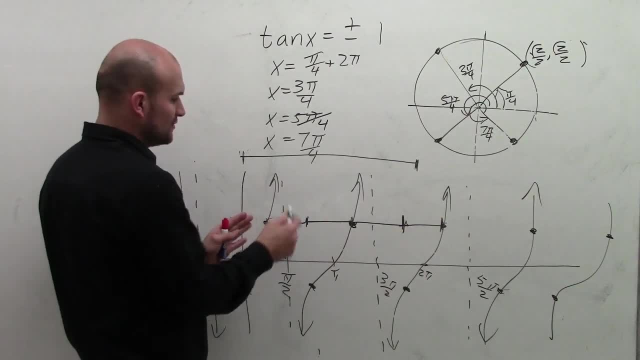 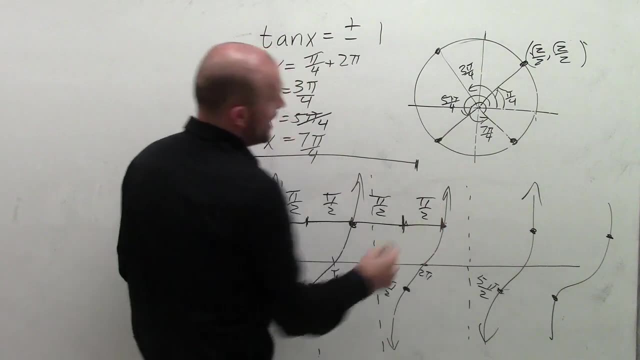 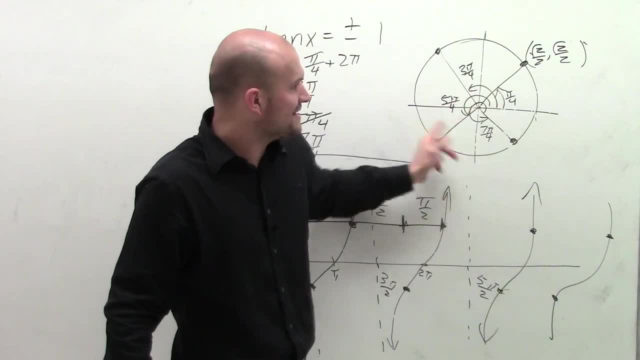 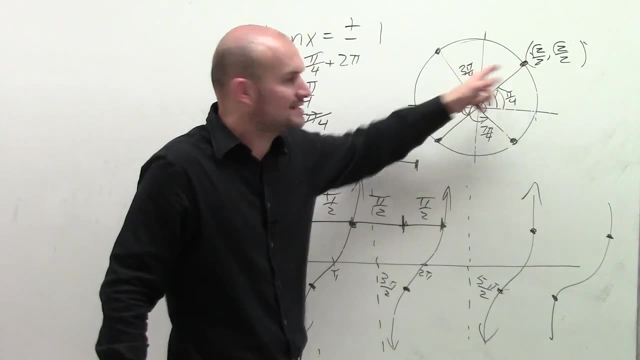 you can also say pi over 4 plus pi Plus pi Plus pi And that's going to cover those two solutions. But why keep on doing it? Why add 2 pi to this answer or even add pi to this answer to get to these two? 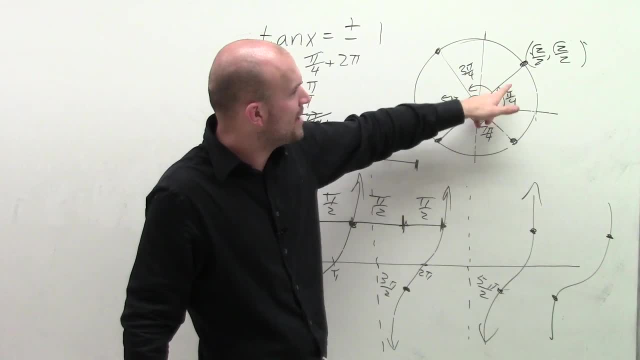 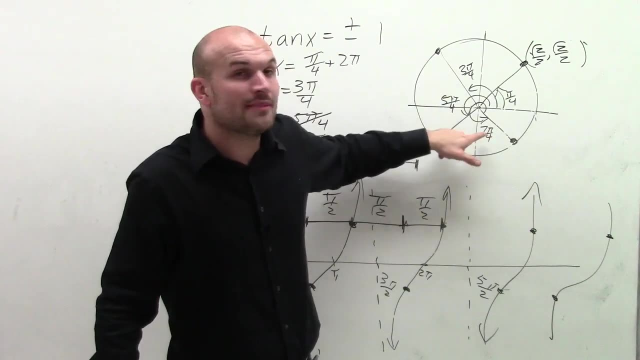 When all you have to do is: if I have this answer, pi fourths. if I add pi halves one time, I get to this answer. If I add it twice, this answer Again three times. this answer Four times.